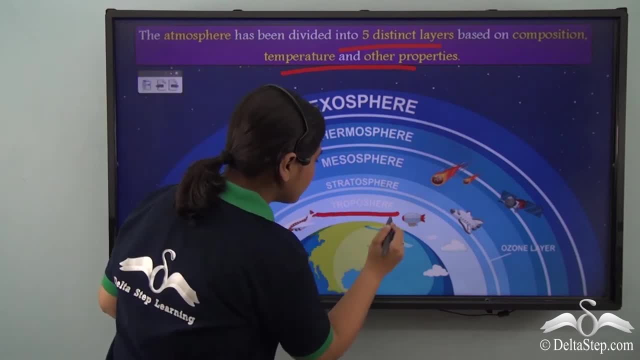 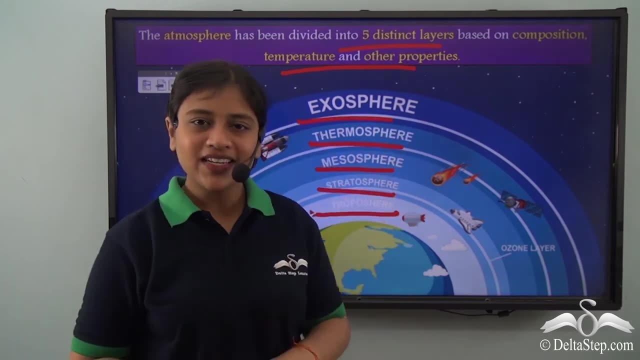 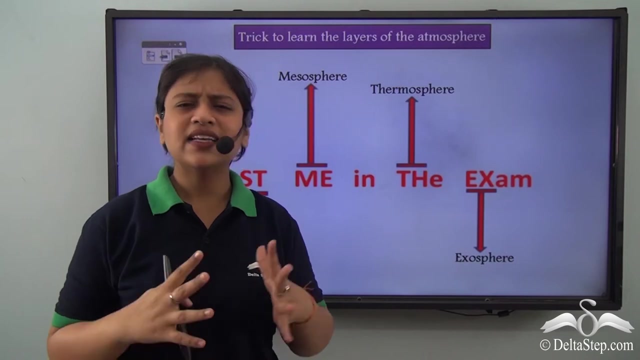 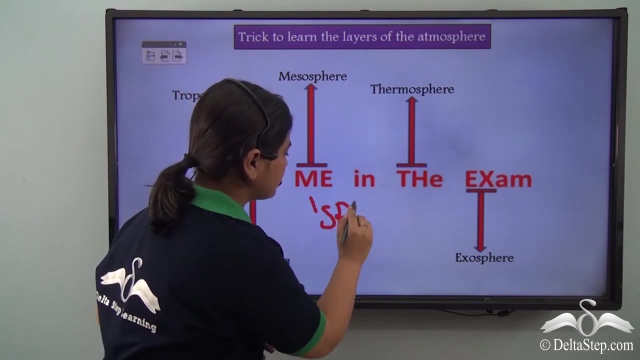 layers? Well, they are the Troposphere, Stratosphere, Mesosphere, Thermosphere and Exosphere, Right, Right, so now that we know that the name of the layers is very similar because all of them ends with the word sphere, Right, But how do we remember them in order? 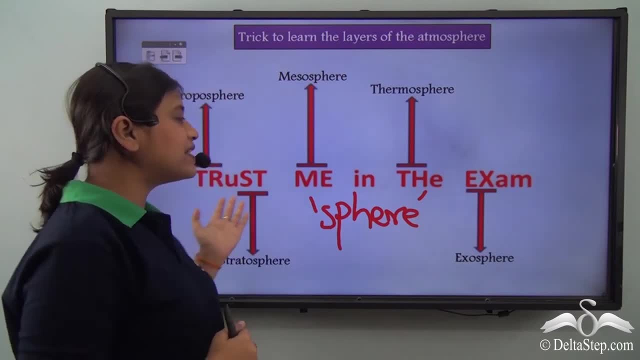 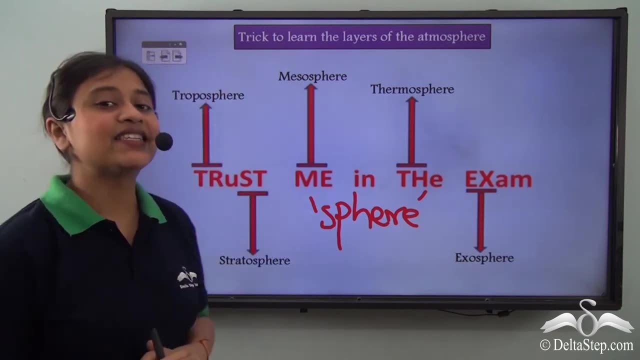 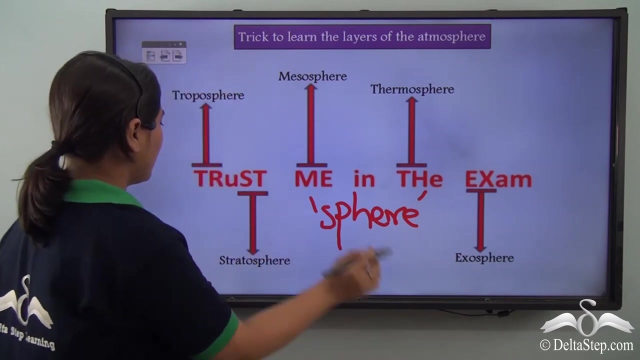 Well, I have a trick for you. This simple sentence makes it very easy to remember the name of the layers in order. So the sentence says: trust me in the exam. So if you focus on the initials, you see that here Trust TR refers to the first layer and that is Troposphere. 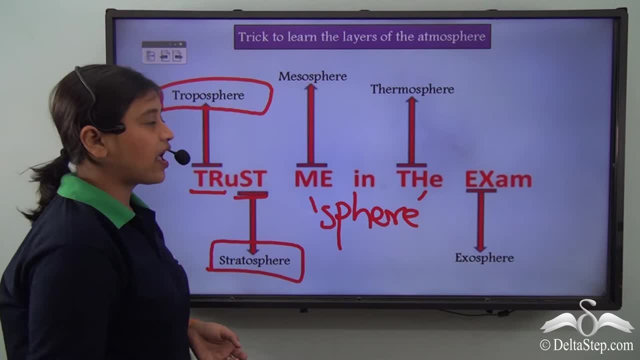 Then we have ST, that is Stratosphere. The third layer here is for Euclidean Trichter, So it seems to be called as Euclidean Trichter. This is that, that which is called Stratosphere. Now, if you see that when we look at the initials, you see that here Trust TR refers to the first. 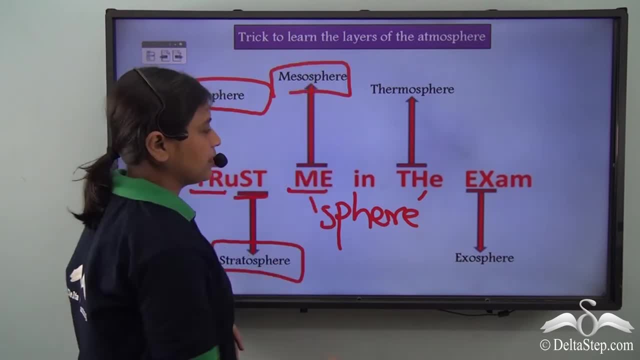 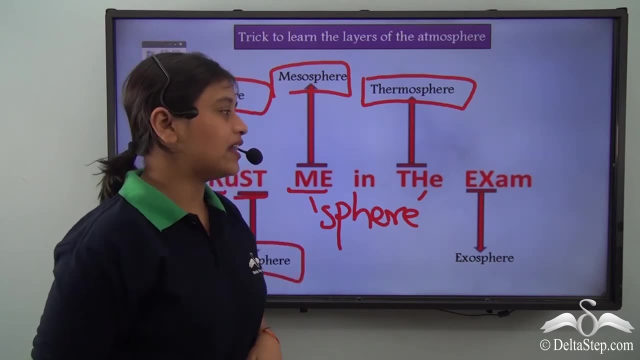 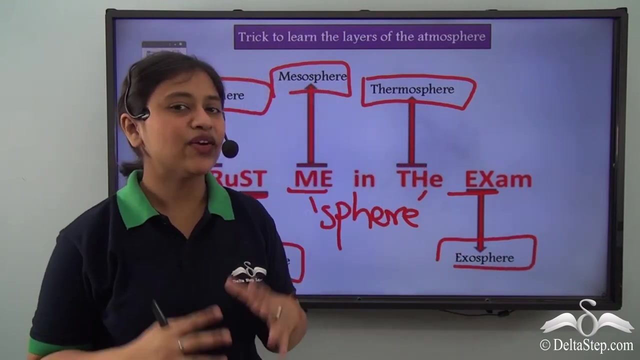 layer, and that is Troposphere. Then we have ST, that is Stratosphere. The third layer here is for ME, that is mesosphere. Moving on to the fourth layer, we have TH, and that is thermosphere, while the last layer is EX, that is exosphere. Right? So this way we remember the name of 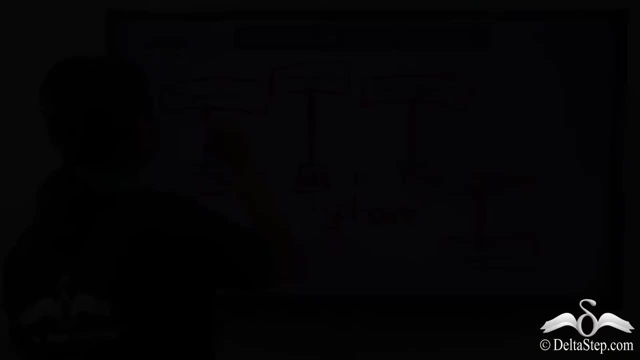 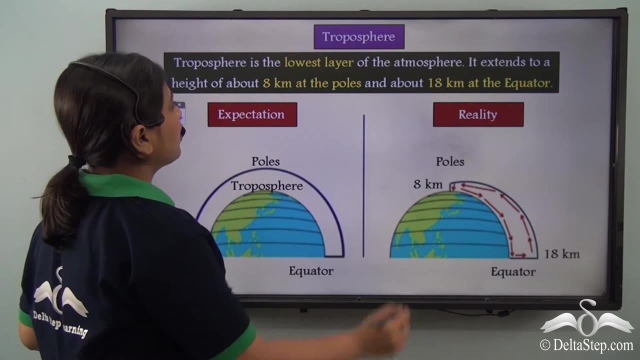 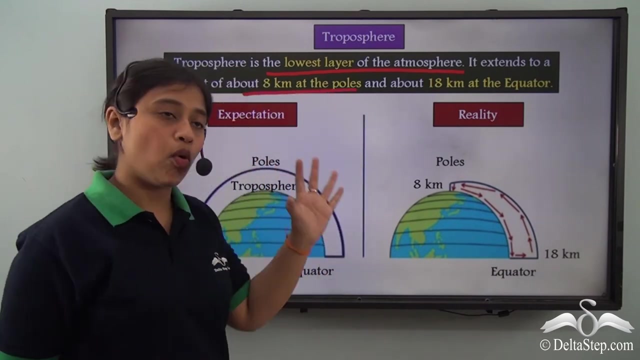 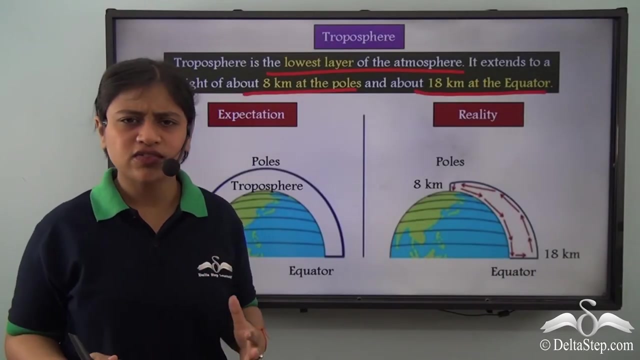 the layers in order. Right, so talking about the very first layer, and that is troposphere, Troposphere is the lowest layer of the atmosphere and it extends up to 8 km at the poles and to 18 km at the equator. You must be thinking that the layers of the atmosphere are uniform. Right, But in reality it extends up to 8 km at the poles while up to 18 km at the equator, So the altitude is higher at the equator while lower at the poles. So what exactly the word troposphere means? Sphere, while we know, is the layer It refers. 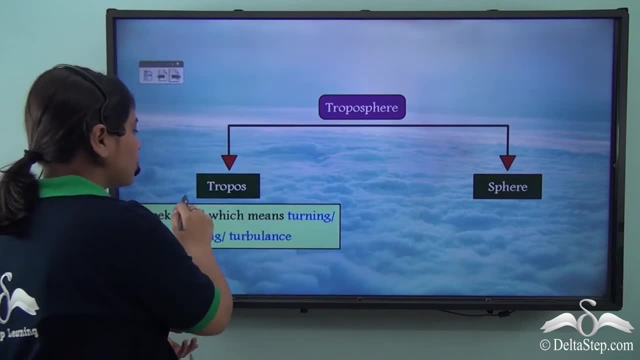 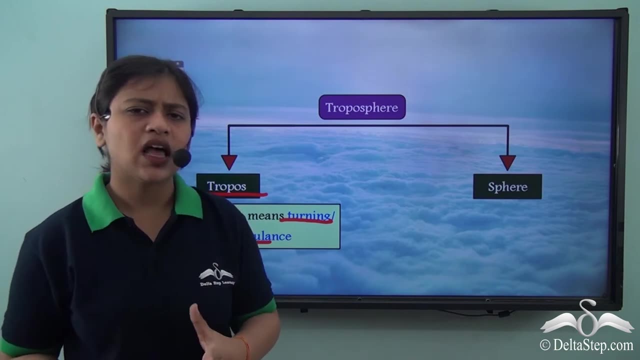 to the layer that we are talking about, While the tropos word is a Greek word which means turning, mixing or turbulence. Now why such a name is given to the first layer of the atmosphere? There is a proper reason. Let's find out. 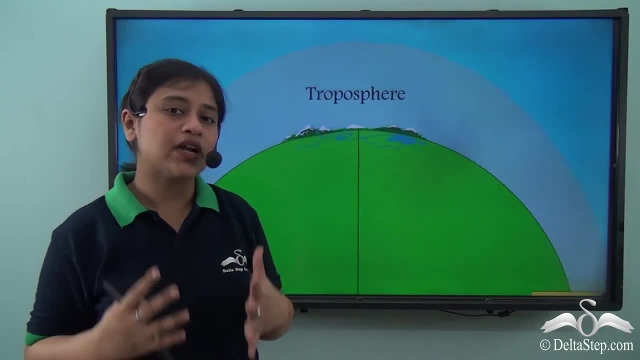 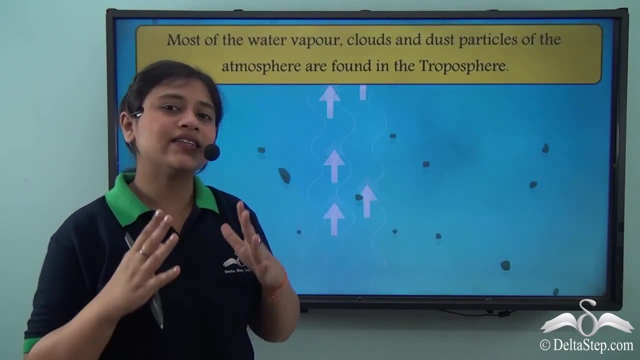 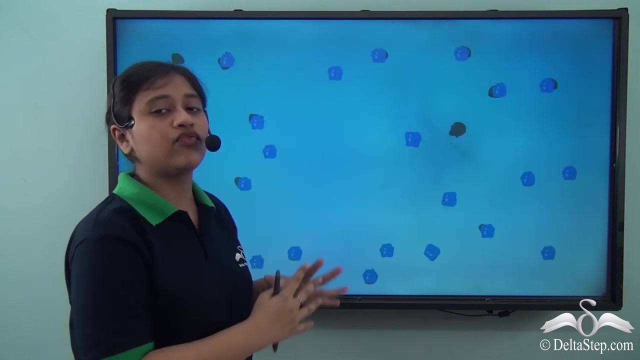 This happens because of the presence of water vapour and dust particles in this layer. The water vapour goes higher into the atmosphere and it condenses on the dust particles to form water droplets. These come together, as you can see, to form clouds. Therefore, this is known as condensation. After that it results into precipitation in the form of rainfall, snow fog, etc. So these weather phenomena takes place in this layer of the atmosphere. Therefore, in the troposphere we have the water vapour and gases like oxygen, carbon. 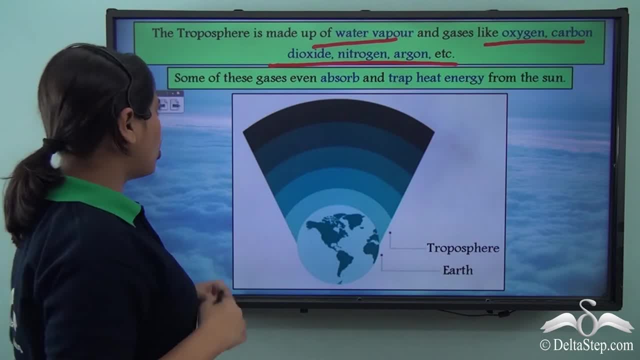 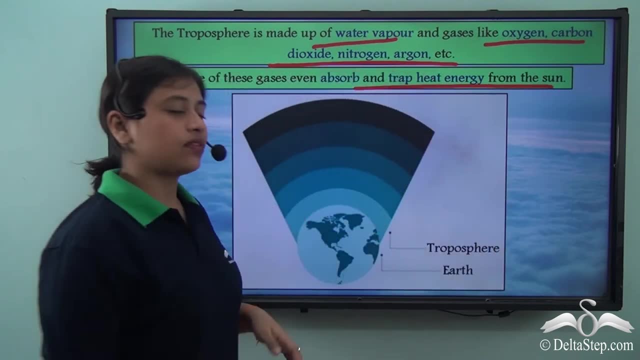 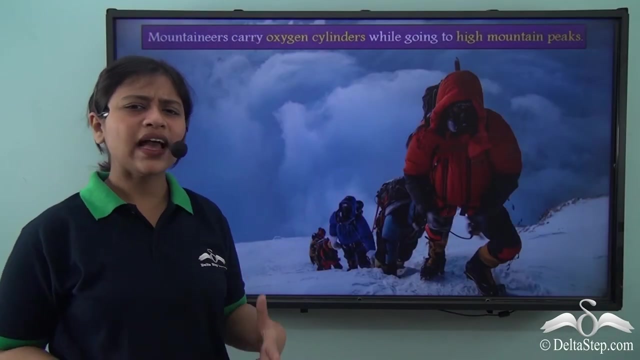 dioxide, nitrogen, argon, etc. Also, some of these gases even absorb and trap heat from the sun. So now here. we learnt about the first layer of the atmosphere, Right? so we've heard that the oxygen that we breathe in is present in the atmosphere. So why do you think that the mountainers carry oxygen cylinders in them? So let's find out. As we climb higher, there is decrease in the amount of oxygen that can cause shortness of breath. So you must have heard about people who are aged or people who suffer from breathing. issues and avoid going to higher rooms. This is because you get struggles on your shoulders when you climb higher with this oxygen cylinder. If you are struggling in the situated places, then get吧 scared. So You must have heard about people who are aged or those who suffer from breathing issues. they avoid going to higher. altitudes. Why is it so? Because of this very reason, The oxygen content is lower at the higher altitudes. Now, why does this happen? This is because of the gravitational pull of the earth. So the gravity of the earth tends to pull down the molecules or the atoms. 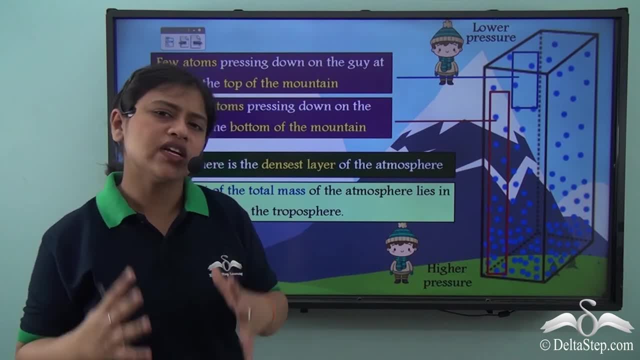 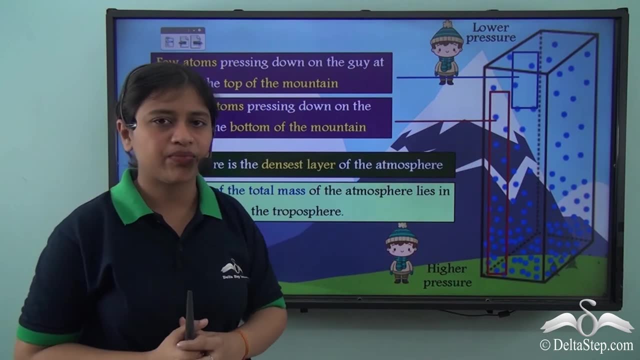 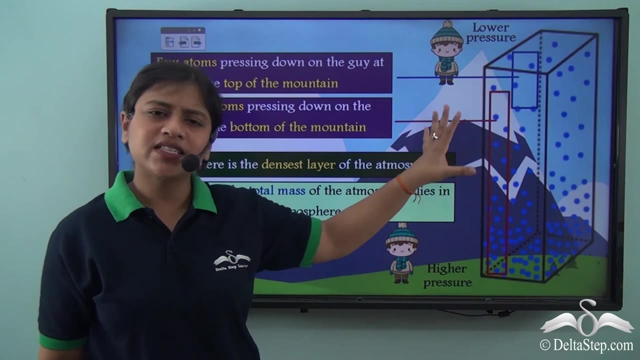 of the gases to the lower layer, to the lower region of the layer. Therefore it is denser at the lower region, while it is less dense at the higher area or at the higher region. So if you look at this guy, you see that there are fewer atoms pressing on this guy at the higher level, while at the lower level several atoms are pressing on him. So we can say that troposphere is the densest layer of the atmosphere, because all the molecules of the gases tend to be concentrated at the lower layer, lower region of this layer. Also, about 75% of the total mass of the atmosphere is constituted. 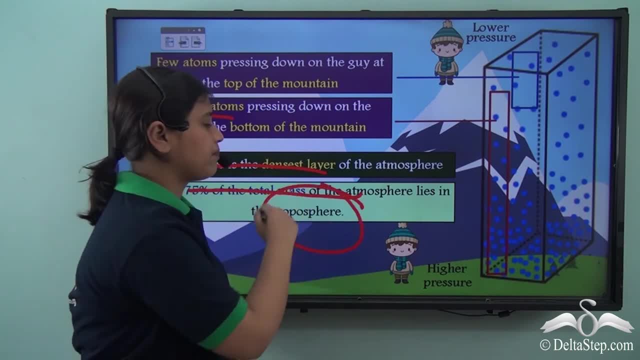 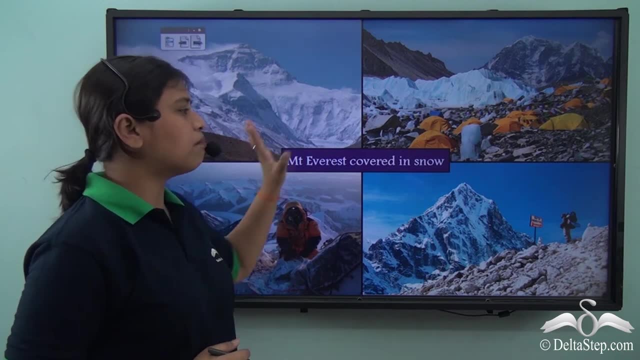 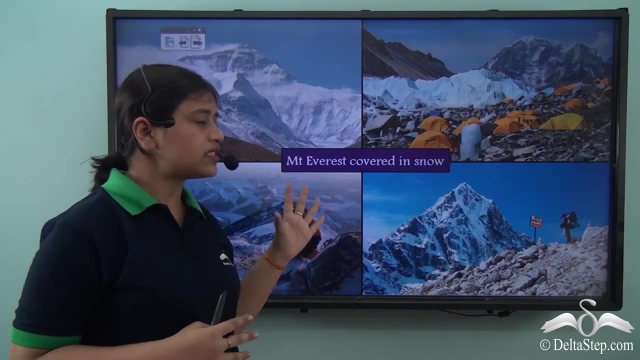 by this layer of the atmosphere that is the troposphere Right Now, as you can see that the mountains are covered with snow. This picture refers to Mount Everest. You must have heard that Mount Everest is the highest peak of the world, So why do you think that? 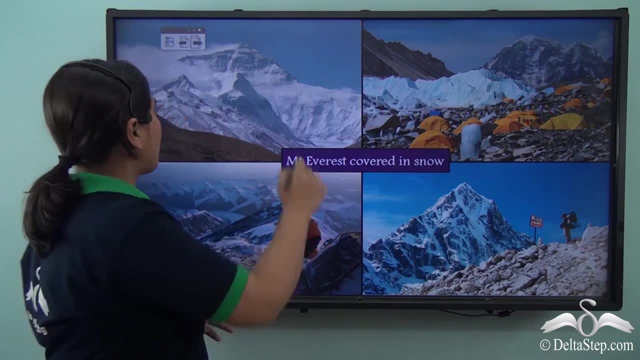 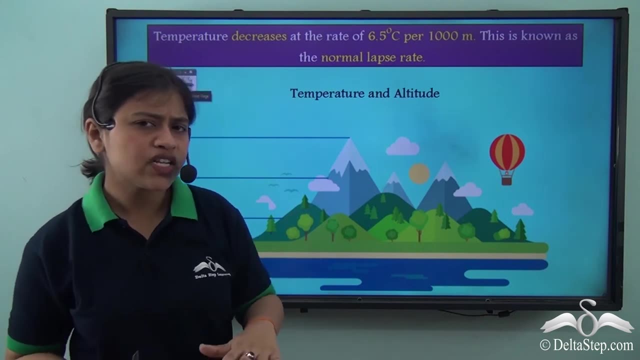 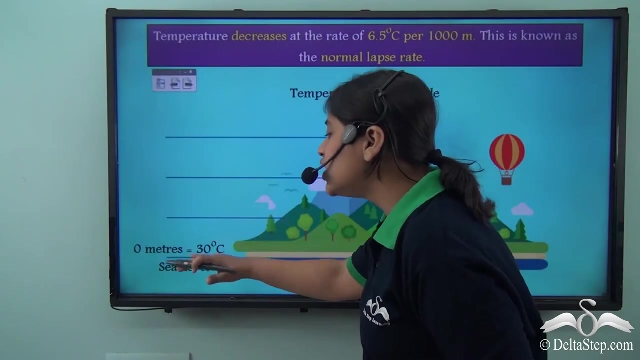 these peaks are covered with snow. This is because of the temperature difference at different altitudes as we go from a lower region to a higher altitude, Right. So what happens? that, if you can see here at 0 meters or at the sea level, the temperature is 30 degree. 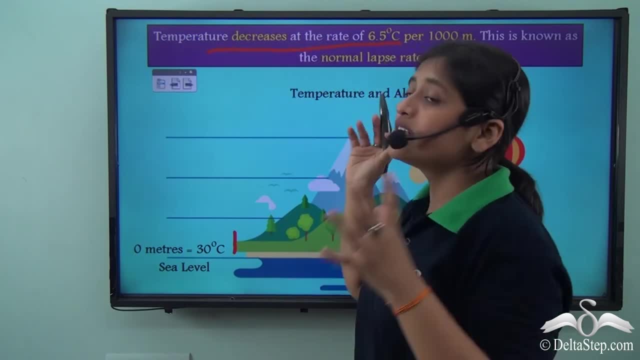 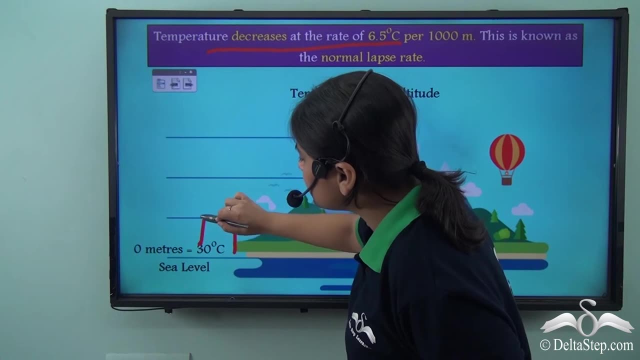 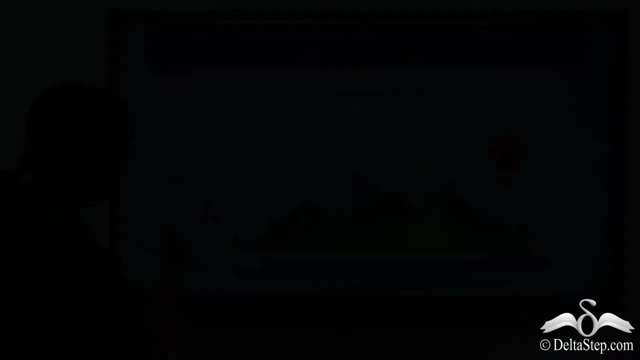 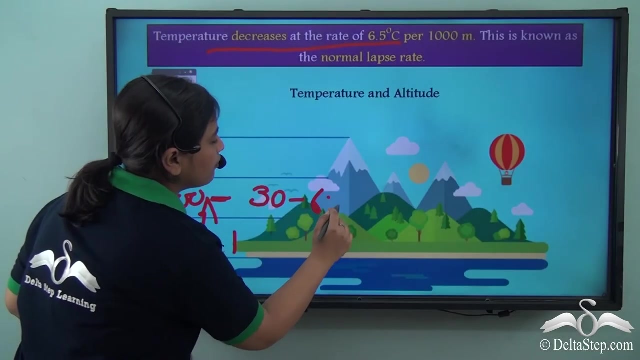 Celsius. So the temperature decreases at the rate of 6.5 degree Celsius per 1000 meter. So if from here we go 1000 meters above, there will be a decrease of 6.5 degree Celsius. So at this level what happens is 30 minus 6.5 degree Celsius will be equal to 23.5 degree. 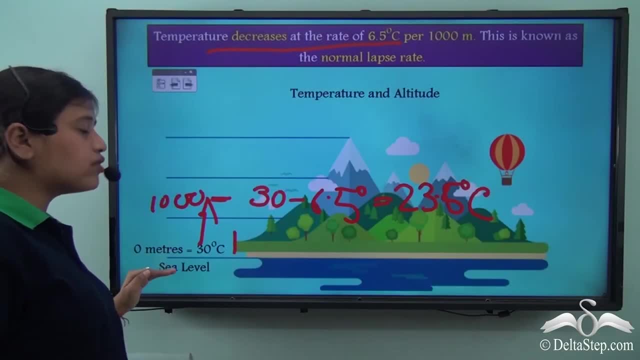 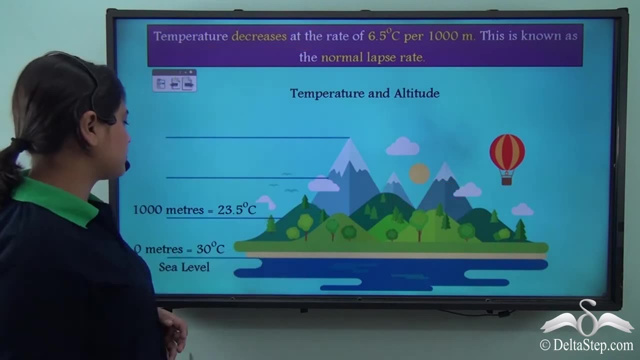 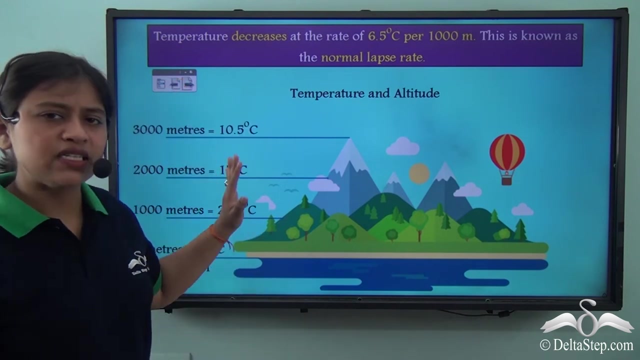 Celsius. So we know that on going 1000 meters above sea level, the temperature will be 23.5 degree Celsius, Right. So as we go higher, 1000 meters, above and above, as it keeps adding, the temperature keeps falling by 6.5 degree Celsius. So at 3000 meters from the sea level, we see that. 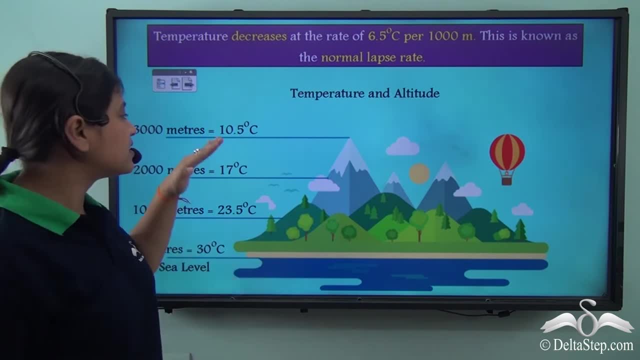 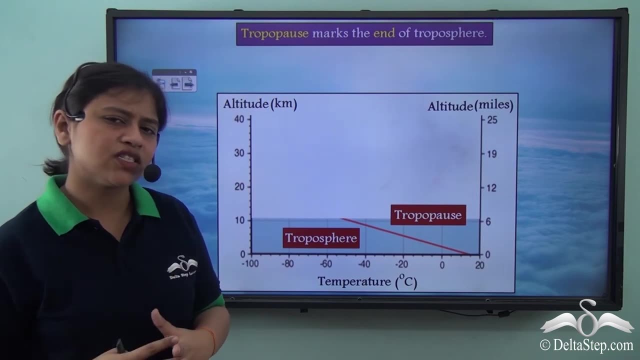 the temperature that was 30 degree Celsius earlier is now 33.5 degree Celsius, So this is a natural phenomenon, so we need to spend some time trying to understand it. The temperature layer is now 10.5 degree Celsius. Now the decrease in temperature happens or keeps going. 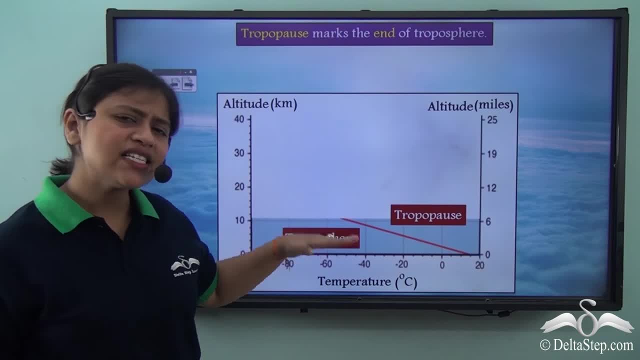 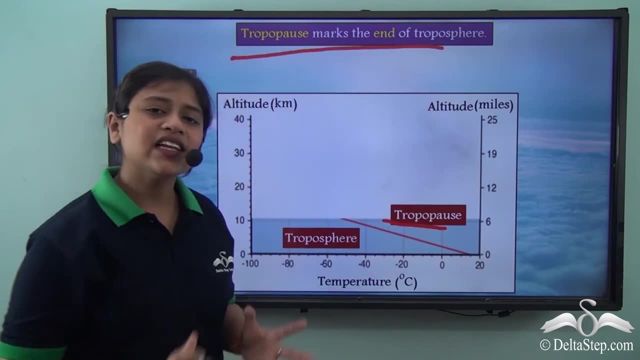 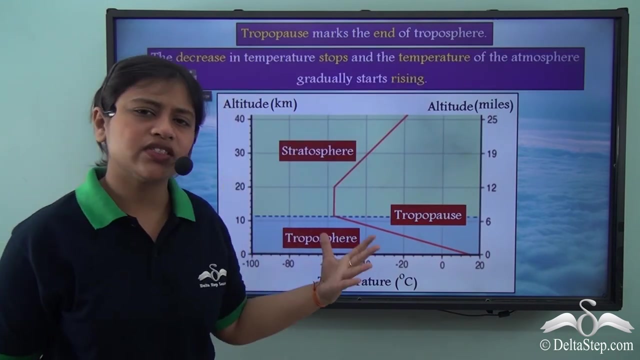 on until we reach the boundary or the end of this layer, and that is called the tropopause. Therefore, tropopause marks the end of troposphere, that is the first layer of the atmosphere. Now, after the first layer, we have the stratosphere, that is the second layer of the atmosphere. 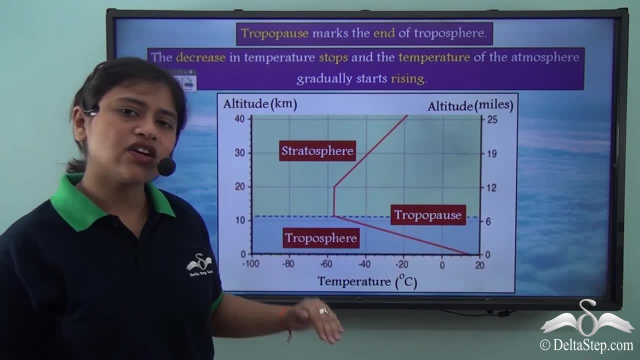 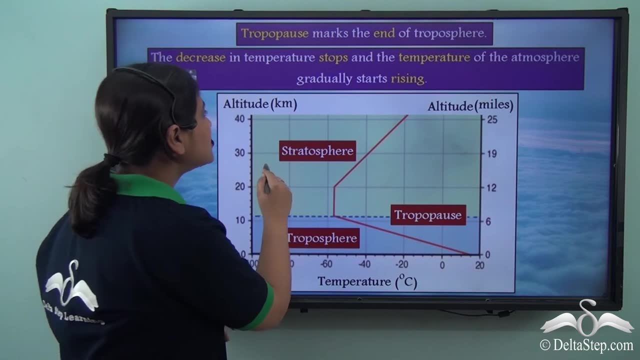 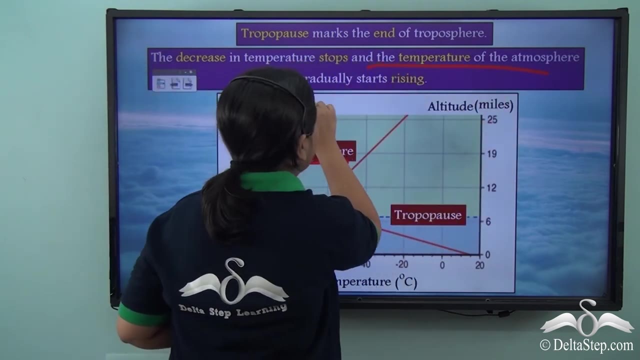 So we can say that tropopause. that marks the end of the first layer, on the other hand also marks the beginning of the second layer of the atmosphere and that is the stratosphere. So the decrease in temperature stops and the temperature of the atmosphere gradually starts. 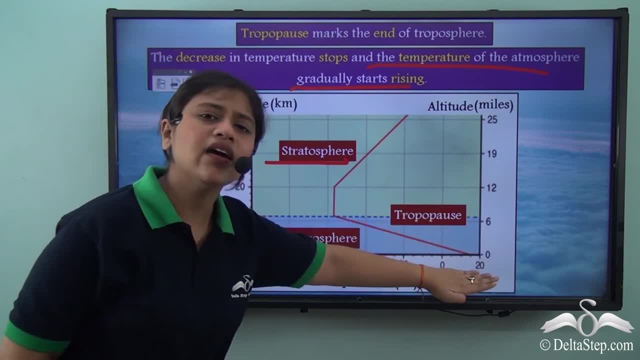 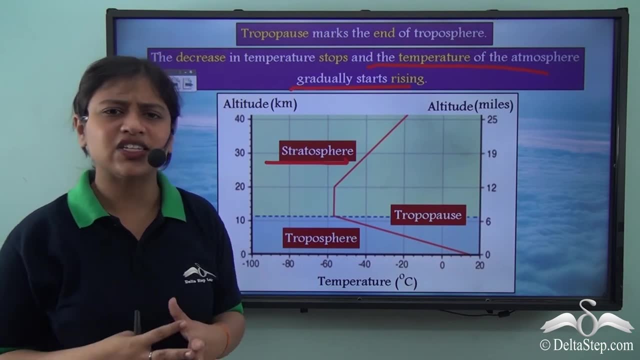 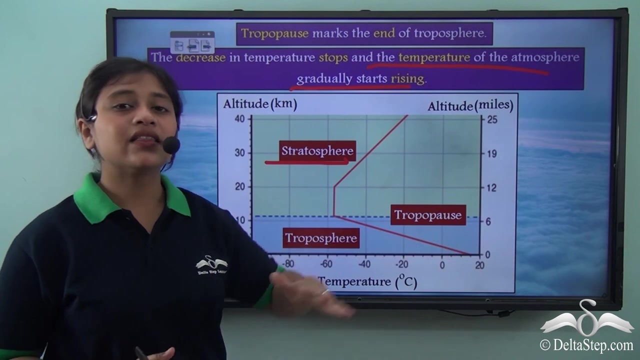 rising. So we notice that as we go higher the altitudes in the troposphere, the temperature is decreasing by 6.5 degree Celsius per 1000 meter. So as it reaches the boundary of the troposphere, that is, the tropopause, the temperature stops. 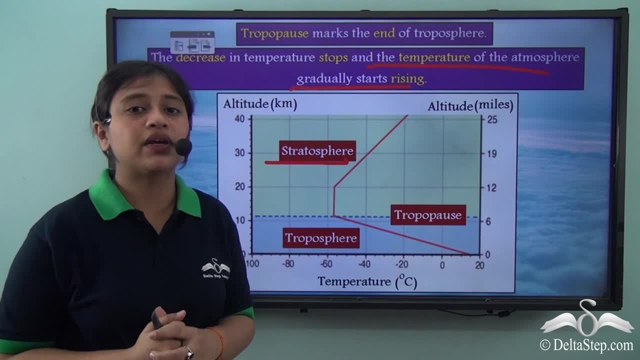 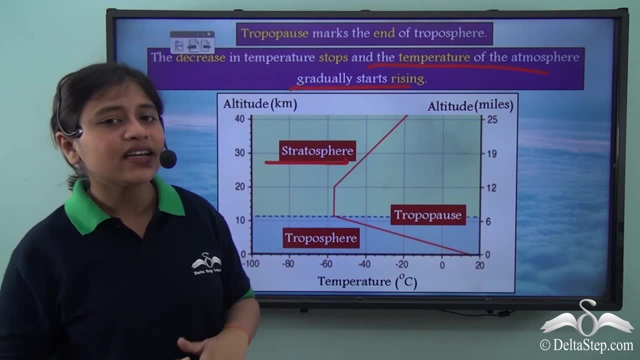 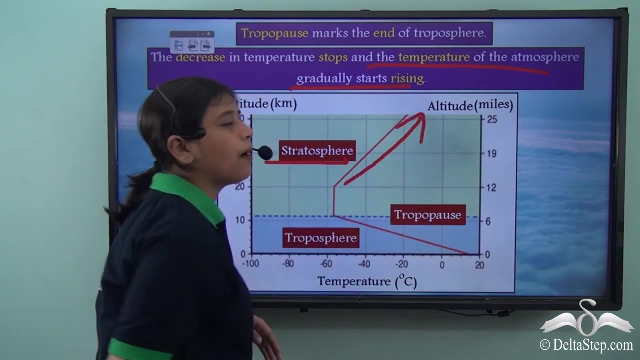 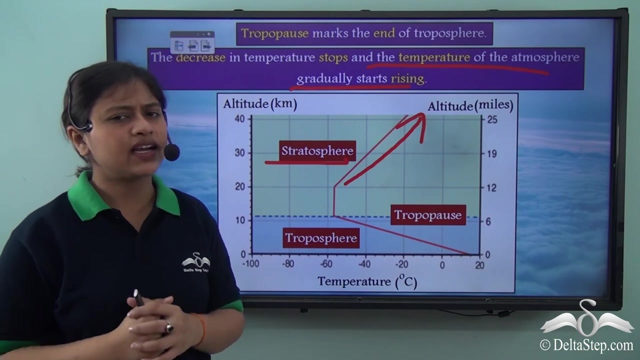 rising or falling. There is no change in temperature. It becomes constant, as you can see. But after some time, as it reaches or enters the second layer of the atmosphere, that is, the stratosphere, the temperature gradually increases. So we see that the temperature fluctuation happens as we change the layers of the atmosphere. 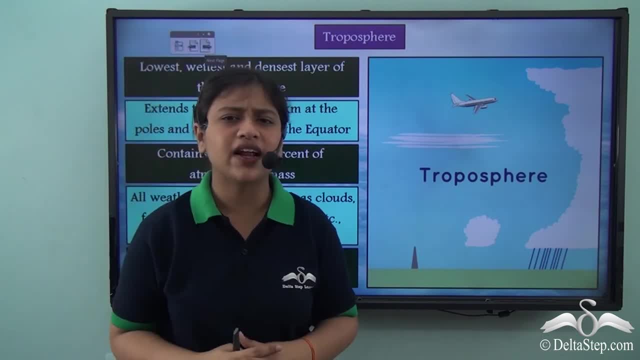 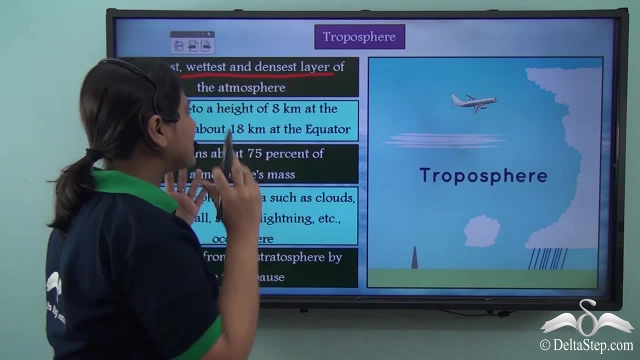 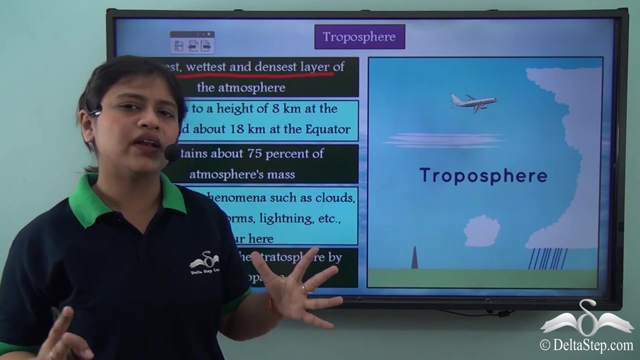 So now let's summarize what we learnt about the first layer of the atmosphere. So the very first point is that it is the lowest, wettest and densest layer of the atmosphere. Lowest because it is the first layer. Wettest because all the weather phenomena